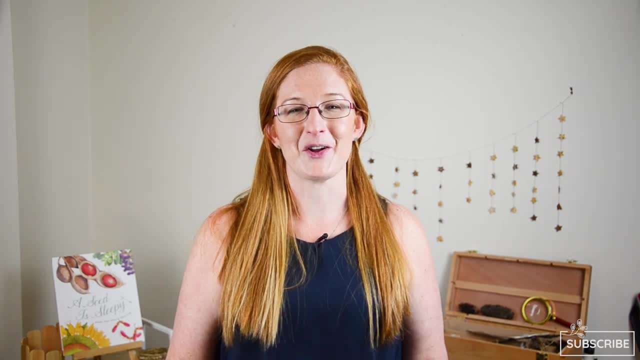 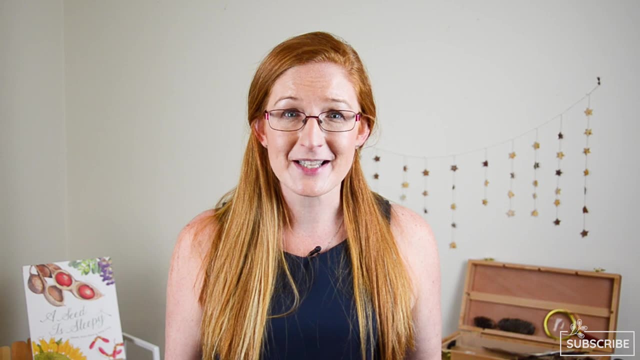 so be sure to keep an eye out for my next video release. It's going to be a lot of fun. All the ideas I'm going to share in this video are super easy to do at home, in your local green space or even in your own backyard. I've got 10 awesome art activities for kids to cover. 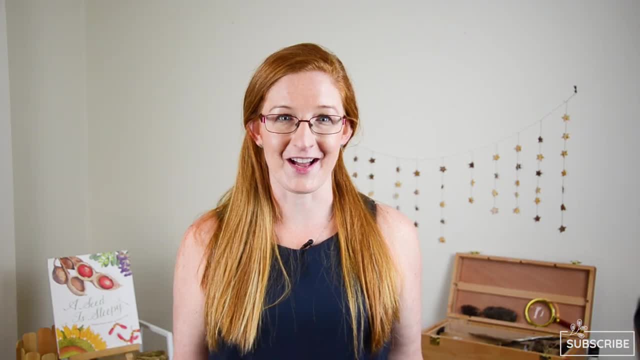 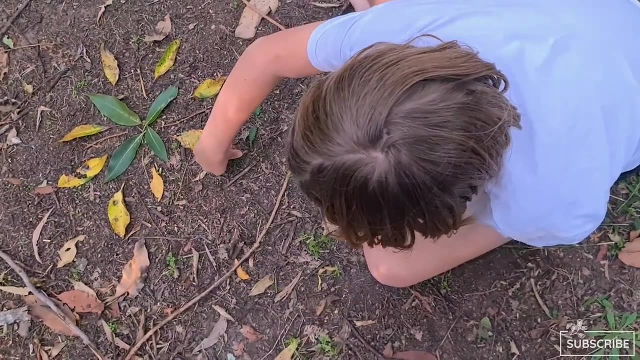 so let's jump in Number one: nature, earth art. For this art activity, explore the backyard with your kids and collect a bundle of natural materials, Lay them out on the damp earth and simply create with them. Leaves arranged delicately can form. 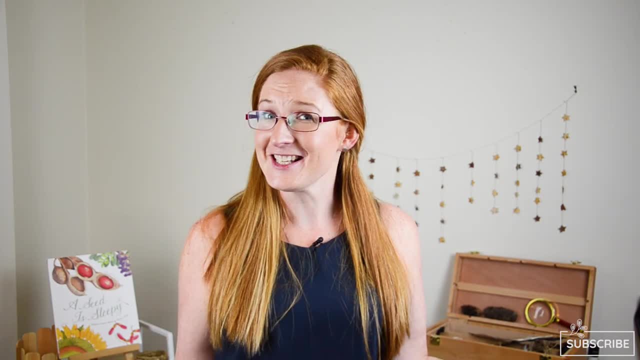 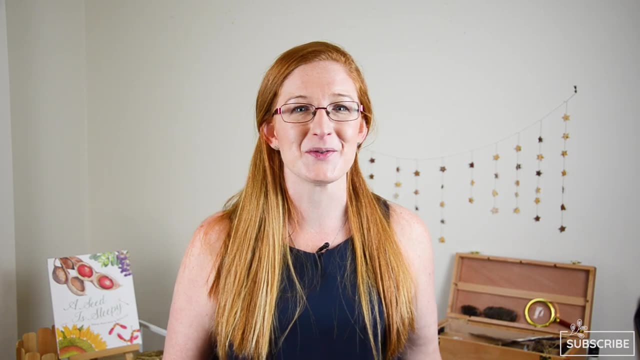 patterns, decorations, frames and creatures and tiny sticks clustered together can become meaningful words. If you want to learn more about nature, play, please subscribe to my YouTube channel, And around them you can decorate flowers, stems, rocks and seeds. 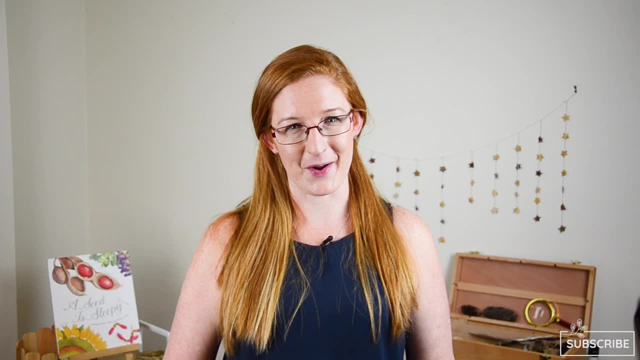 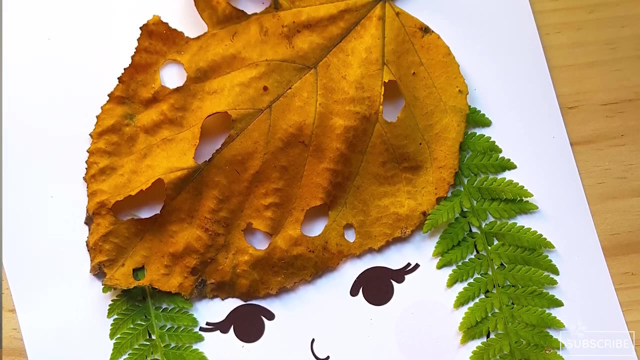 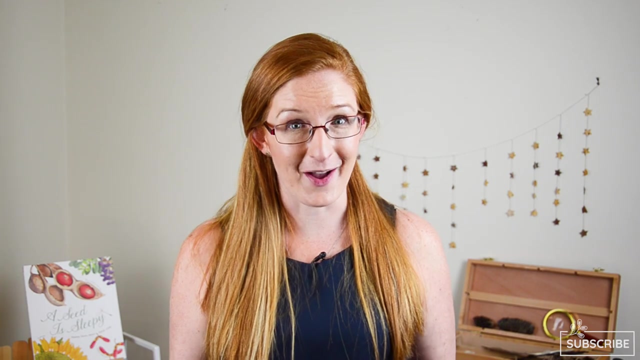 which all add colour, texture and depth to artworks. If your kids love nature collages, they might also enjoy this free Nature Head printable. You can find the link in the description below. Number two: painting with natural materials. Your children might relish in the labour of. 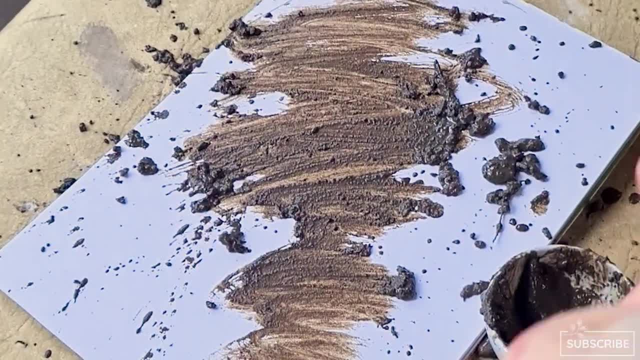 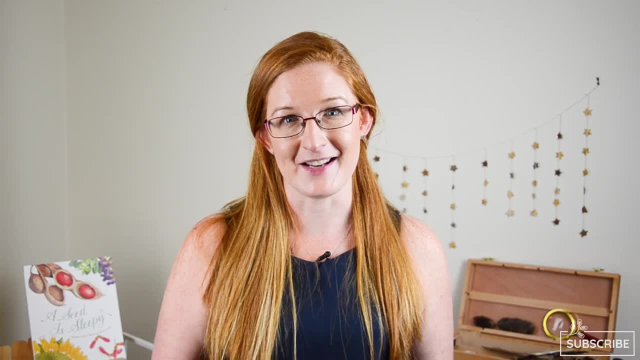 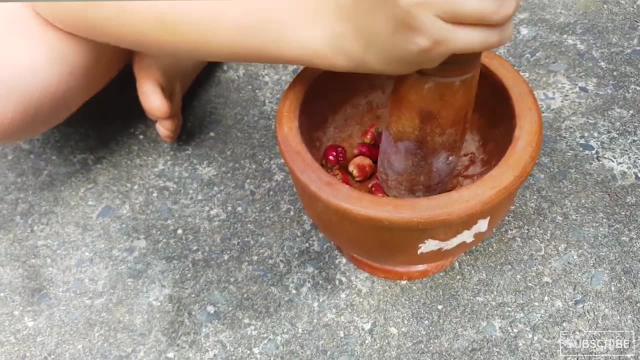 making their own painting media before the creativity truly begins. For example, combining dirt and water together will mix different shades of brown paint, and using a mortar and pestle to bruise flower petals or leaves creates juices to add an earthy colour to their paintings. 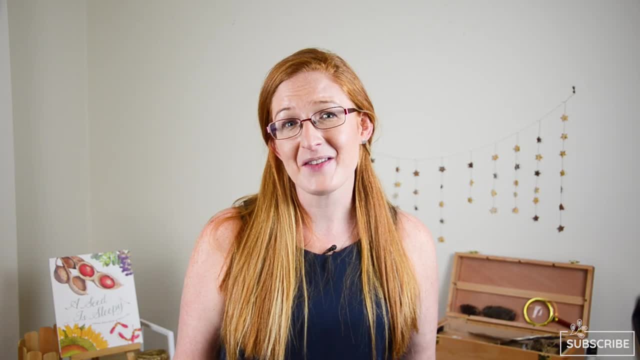 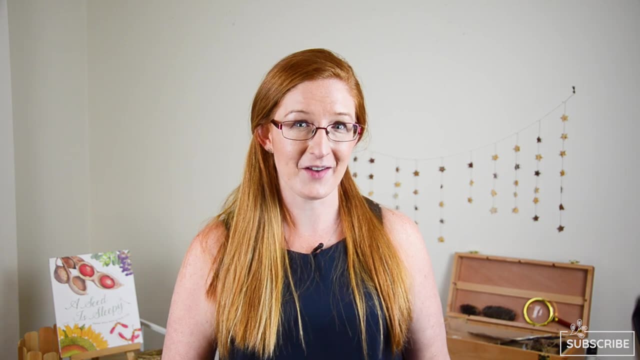 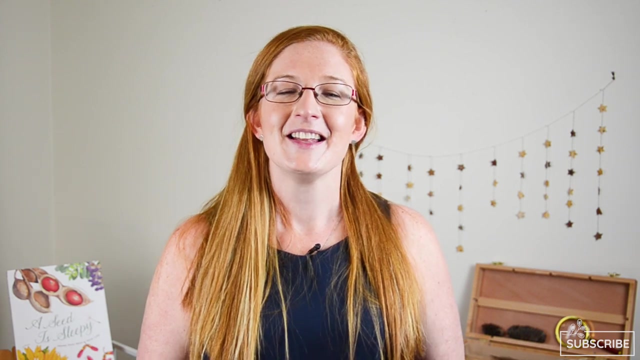 The process will be so lively and diverting they may forget to paint their creations altogether. Of course, they may also be so inspired by the handicraft that they spend more time on their masterpieces too. If you're enjoying this video, please consider giving it a like. This helps me to reach other 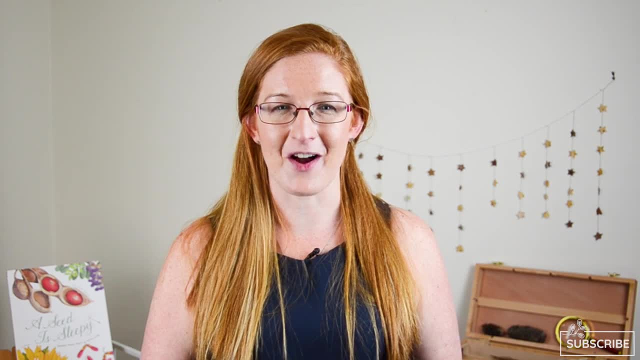 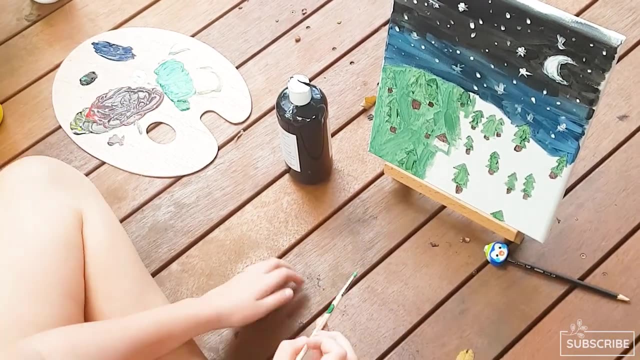 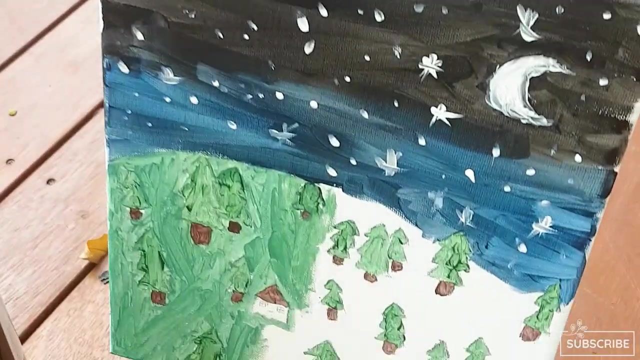 parents and continue getting more kids outside enjoying time playing with nature. Number three: nature portraits. Most children have been asked to draw something from nature before. Perhaps they were invited to sketch the world on Earth Day or paint a koala during Save the Koala. 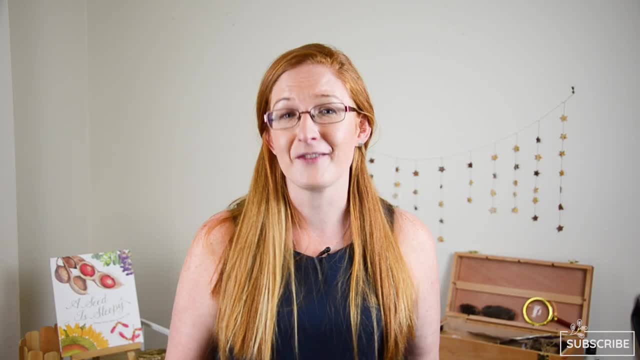 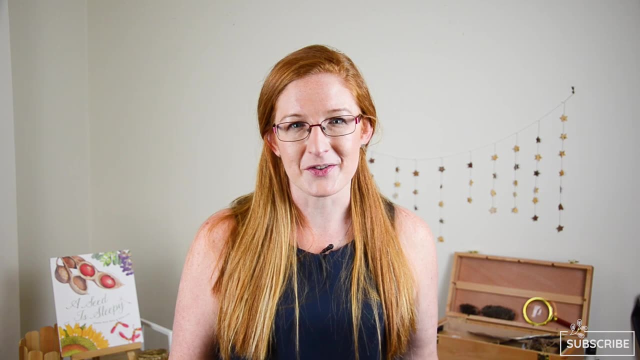 Month. But drawing something that you were told to draw can feel very different to something that you see and feel connected to in nature, something that you get inspiration from all by yourself. The simple act of your child creating art outside is enough to inspire their art to look. 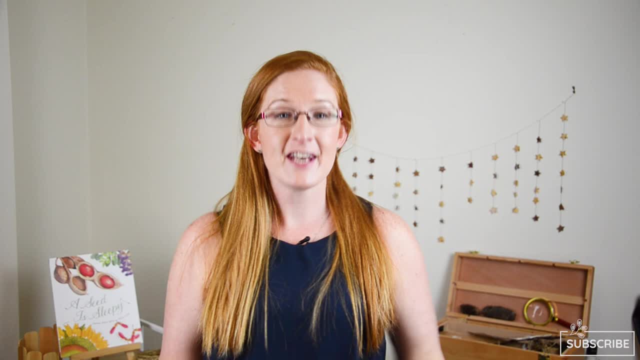 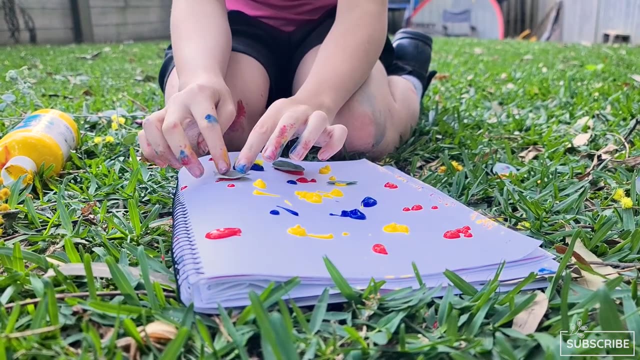 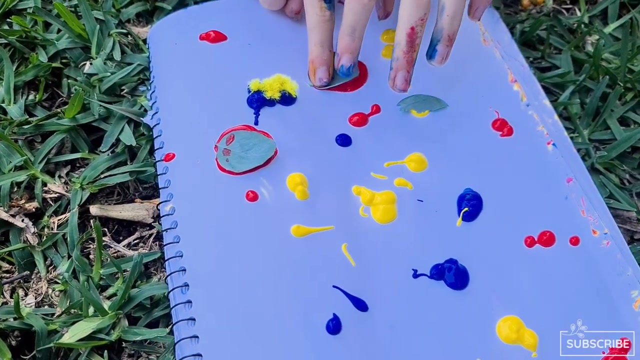 and feel different from anything they might have produced before. Number four: nature collage. Nature collages are a favourite of ours. Our artwork can seem a bit dull without the added texture created by a cluster of seeds on the canvas, you know, or some tiny twigs that are assembled to bring the image out of the flat surface. 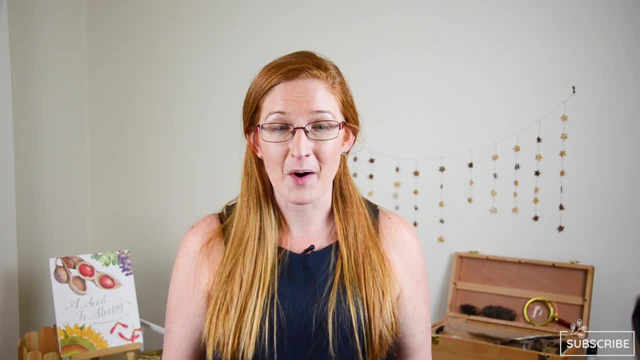 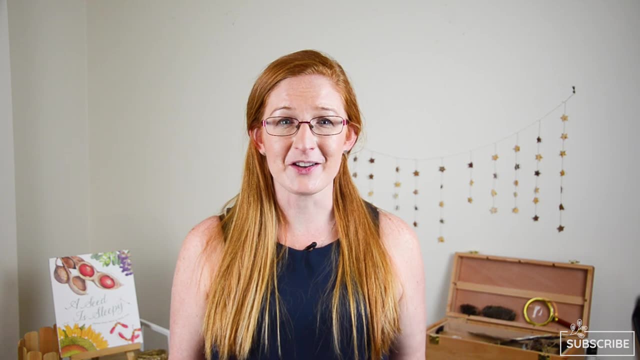 So collect a heap of natural art materials from the garden and combine them with the media that you tend to use with your kids, like paints and crayons or pencils. Your kids will soon realise how nature allows their artworks to splendidly pop off the page. 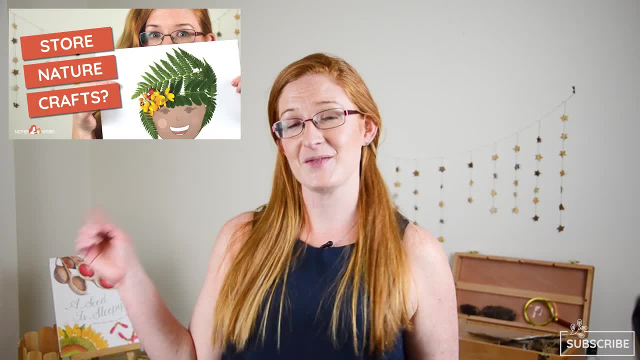 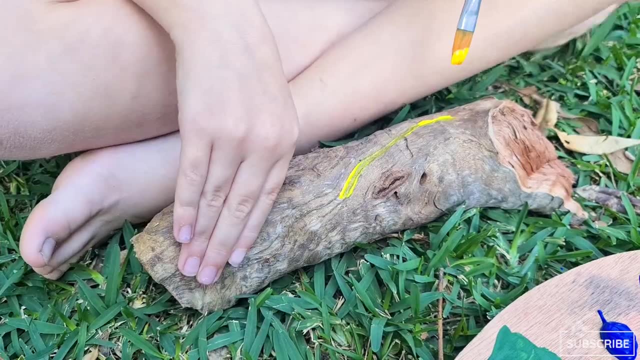 If you would like to learn how we store our nature artworks, head over to this video. next, Number five: painting on natural materials. My next suggestion is to make nature your canvas. Painting items on natural materials has occurred for thousands of years, and it's only natural to. 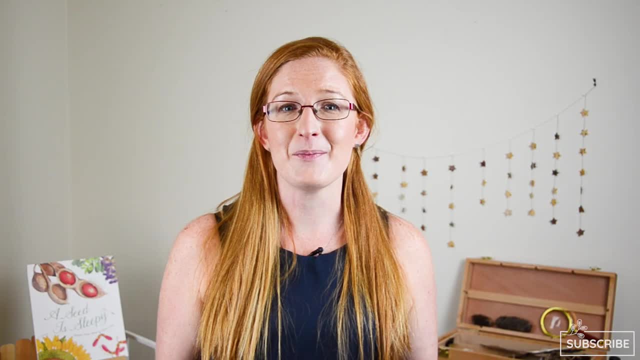 feel at home when you're painting on your canvas. So if you're looking for a way to create your own art, you might want to start with painting on a rock, a leaf, a seed pod or even a flower. So send your kids out and see what they might like to paint on next. 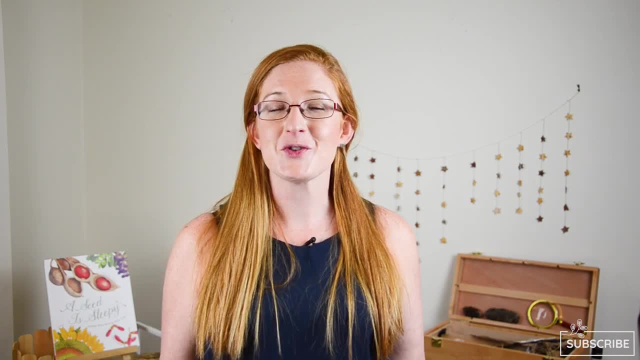 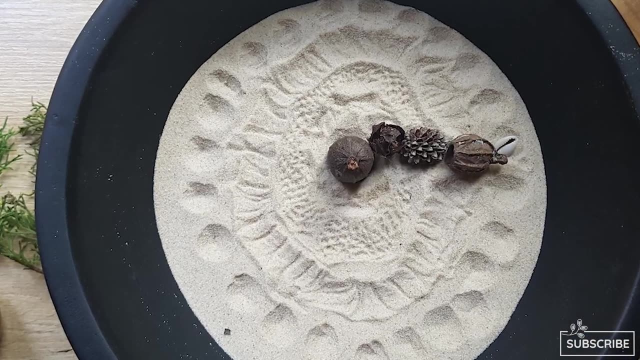 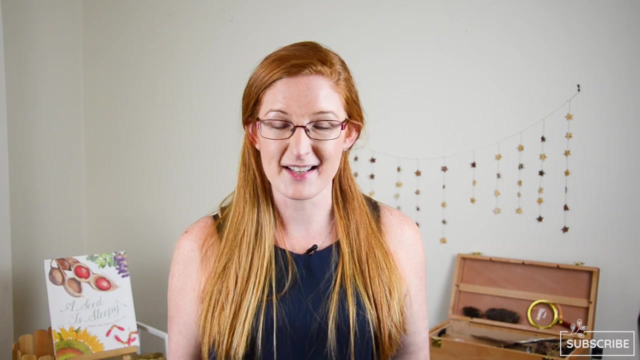 Number six: sand art. There is something so relaxing about creating art with sand, and I gave this natural material a section all to itself because it's incredibly therapeutic, especially when used in art. So, keeping artwork simple, children can form patterns and shapes in the sand, or make art using sand itself. 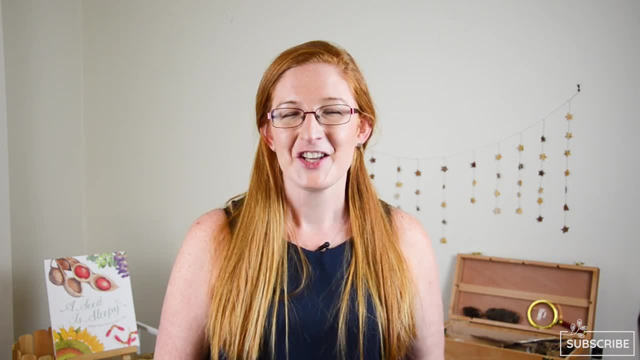 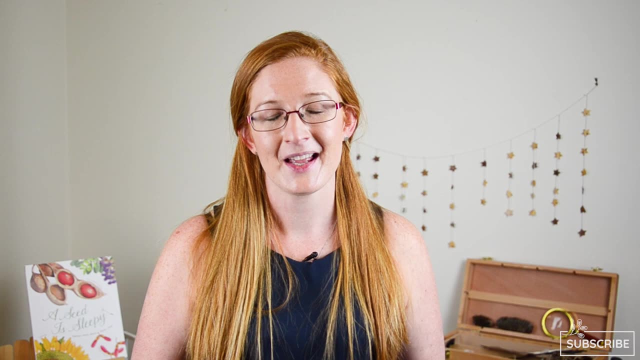 They may only need a paper and a glue stick and a bit of sand to create their own artworks, And, of course, I'd suggest that you add sand to the artworks that I've already mentioned too. Number seven: nature photography, If your child isn't entirely comfortable getting creative with. 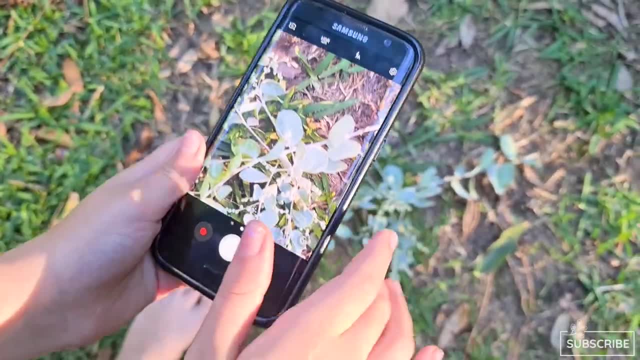 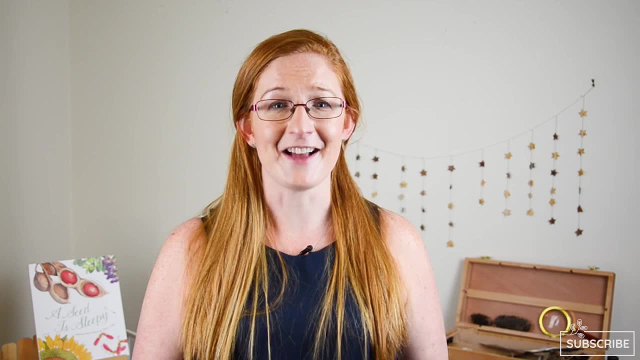 natural materials, you may find that they are more content behind a camera lens, focusing on a subject in nature and trying to capture it. Nature photography is art and learning the basics of photography may be a bit of a challenge, But if you're looking for a way to create your own art, 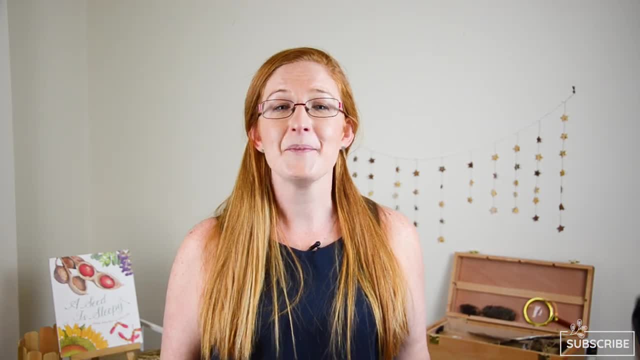 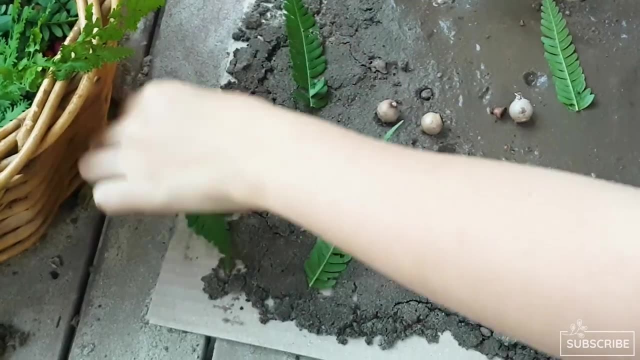 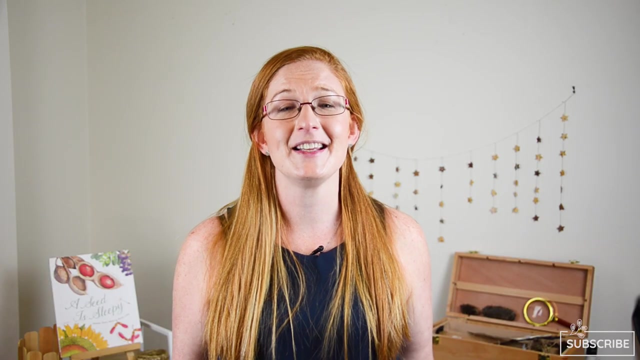 nature photography may be just the creative outlet your child needs. Number eight is mud collage. Now, my girls have spent a lot of time in their mud kitchen. This is a creative escape all on its own, but recently they've begun creating their own mud collages, and it's really lovely to watch them create. So imagine dirt and water. 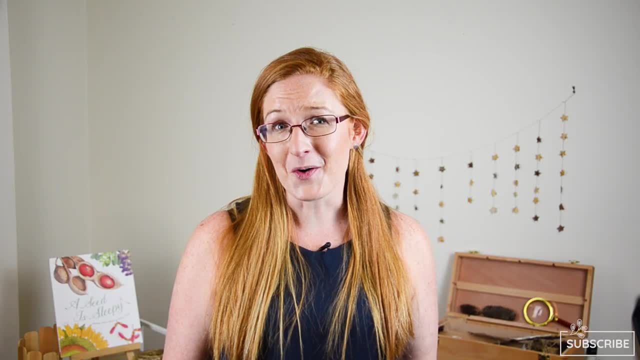 muddy hands and botanic decorations. Best of all, they were able to watch their artworks change as the mud dehydrates. So imagine a lot of mud and water, muddy hands and botanic decorations. Best of all, they were able to watch their artworks change as the mud dehydrates. 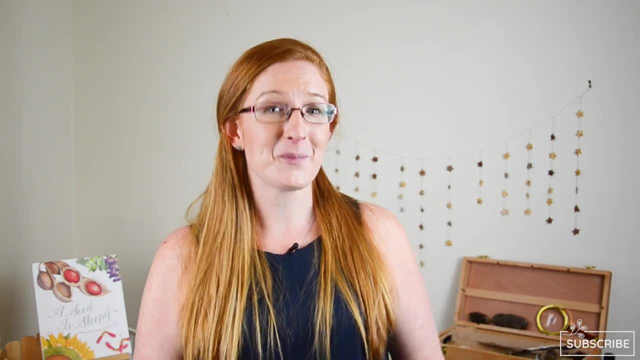 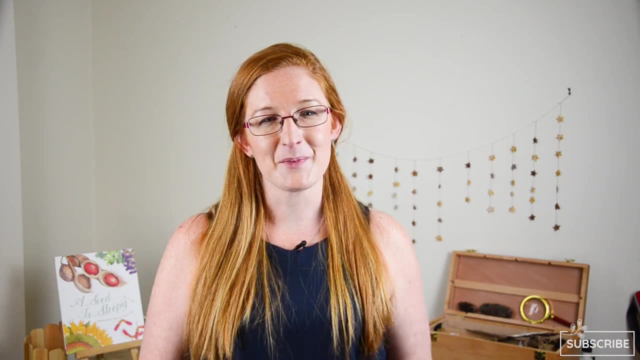 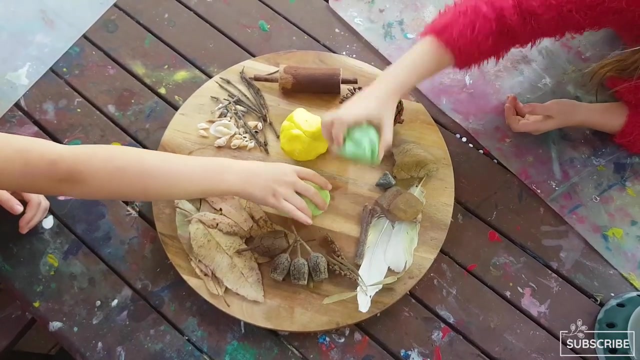 Each day. if you would like to see more ideas for playing with mud, I've done a whole video for that purpose. I'll add the link to the description below. Number nine is Plato and nature. When used together, Plato and nature combined become a beautiful, open-ended art activity for kids. 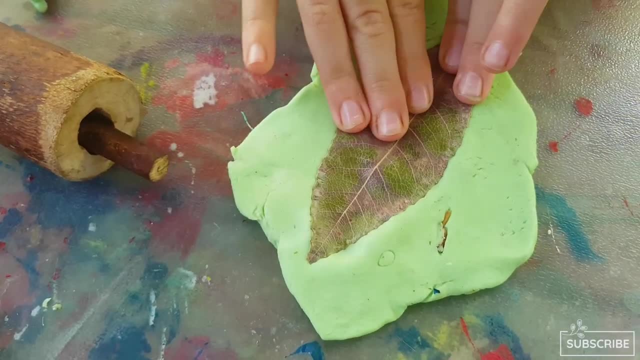 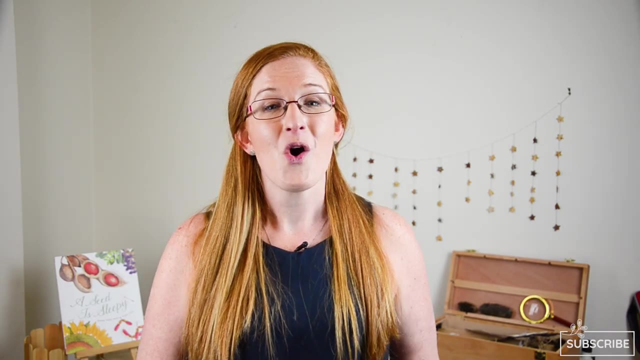 Place everything on the table and watch them shape, form and design with all the materials at their fingertips. They might give life to textures, form patterns from the natural materials or construct sculptures. It's important with this activity to just let them go for it in whatever. 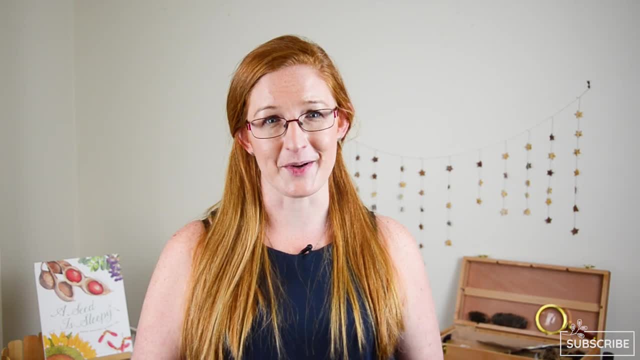 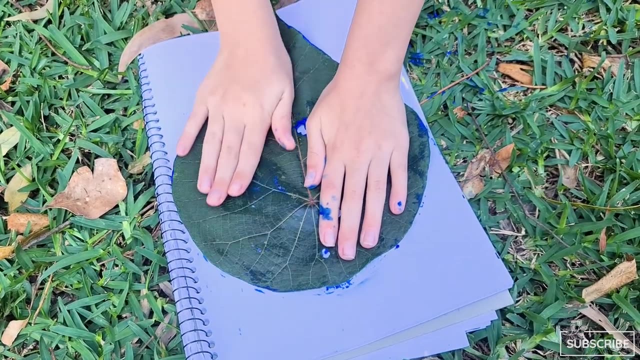 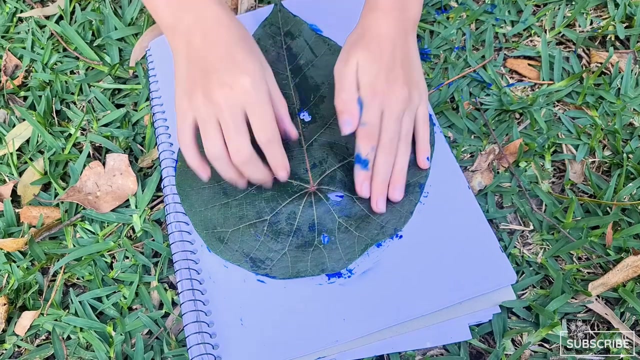 way inspires them. Number ten: nature prints. The simple exercise of painting a leaf and pressing it onto paper and running your hand over the top is a sensation that's hard to explain. There's a level of expectation and surprise as you gently but quickly fold the leaf off the paper to expose. 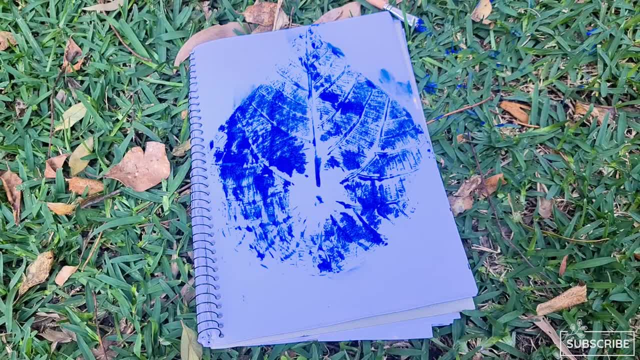 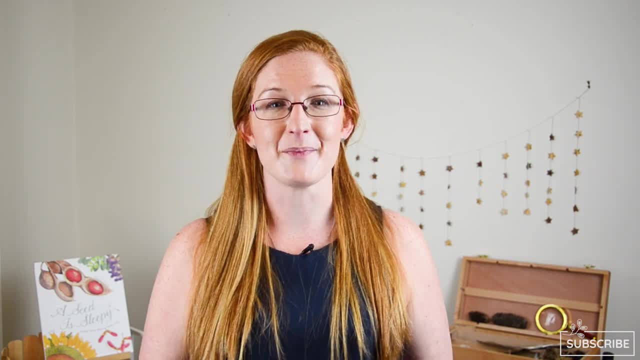 the patterns of veins underneath. If your child is young, you might like to show them how to do it And then let them do it themselves. But if your child masters it quickly, you might like to suggest making this leaf softy. Don't forget, you can use other materials too to 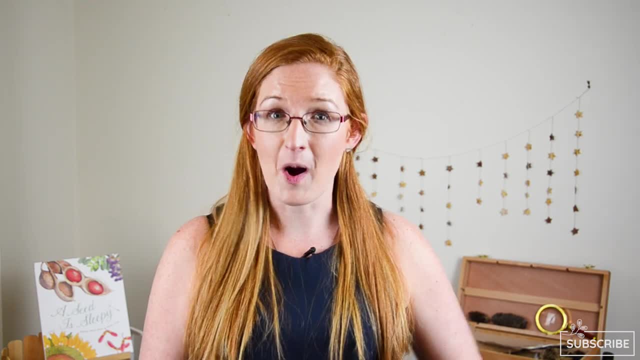 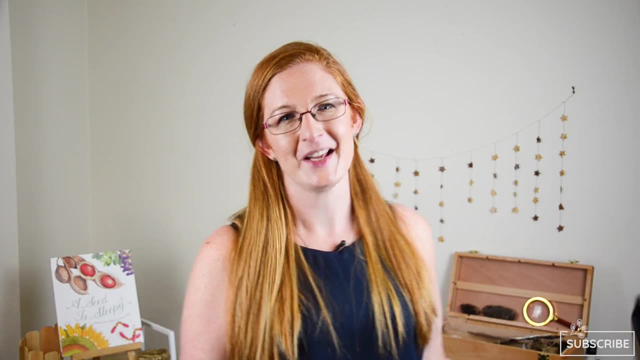 make nature prints. You can try gum, nuts and rolled pine cones over the paper with paint and seed pods as well. Number eleven: I know I said ten, but this one's kind of cool too. So make nature paint brushes. Make your own paint brushes with nature and create a masterpiece. 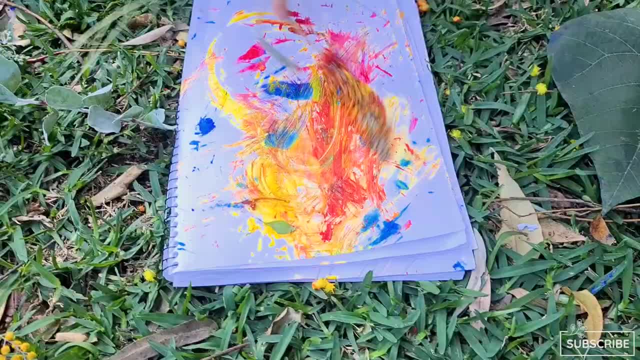 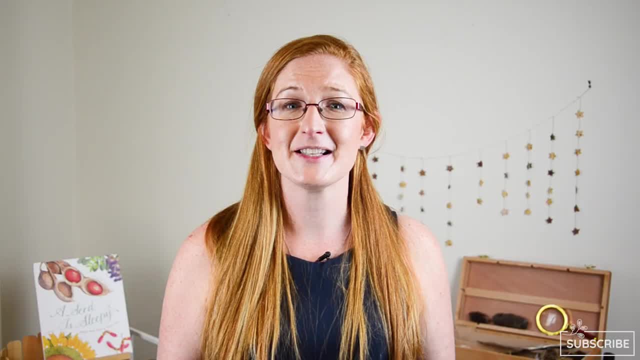 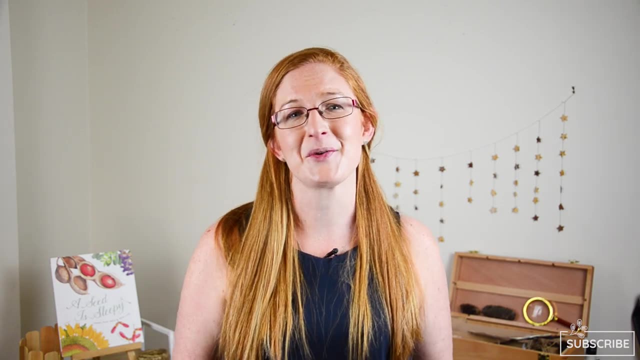 painted solely using the natural endings you secured on a stick. I can safely say that it is a lovely way to help your child let go of perfection and realism in art and embrace abstract uncertainty on the page. Use grass, leaves and flexible twigs to create your own paint brushes Your kids will love experimenting with. 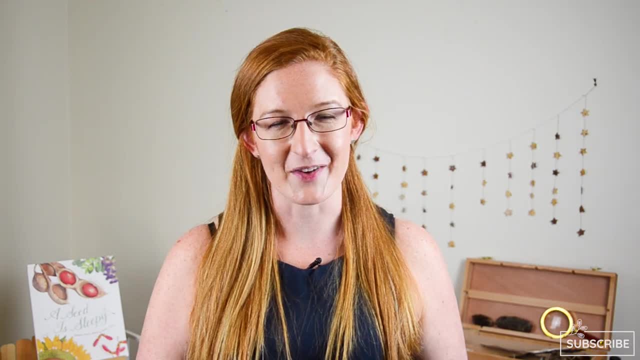 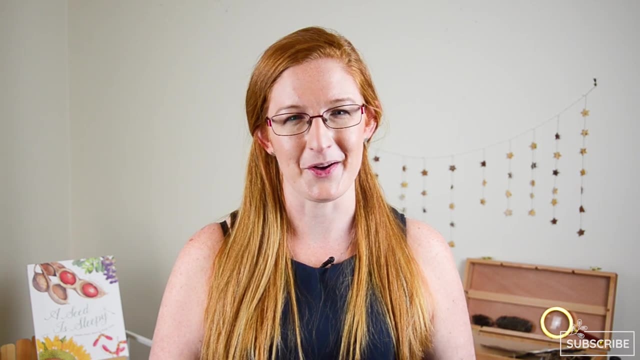 these tools. I hope you enjoyed all these nature art ideas for kids. If you liked this video, please go ahead and let me know which one you love the best and put it in the comments below. Again, if you would like to get more nature art videos like this, please subscribe to my channel.